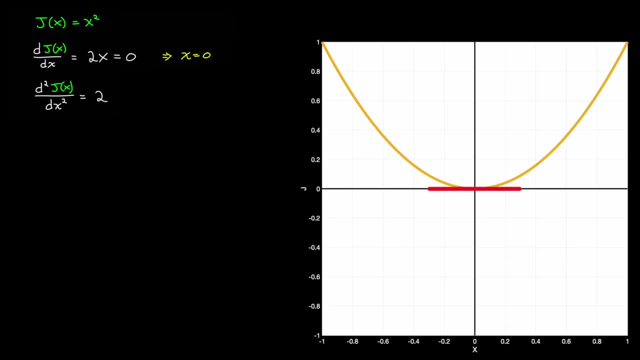 that derivative equal to zero, And then we can determine that the rate of change of the slope is positive by just looking at the second derivative at this point. Now, similarly, we can show a maximum point for j equals negative x squared, since the second derivative is negative, And 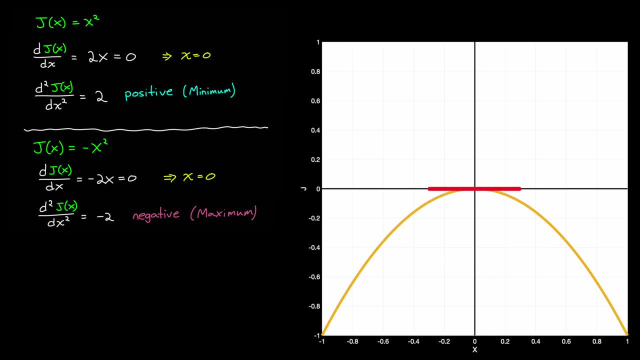 therefore, we can deduce that the output is curving down. from this one point, x equals zero. And then, finally, we can show that the flat part of j equals x. cubed is neither a maximum or a minimum point, since the second derivative is zero. at this point It's neither positive or negative. 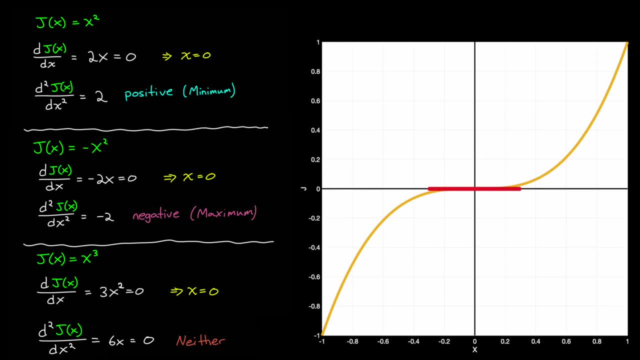 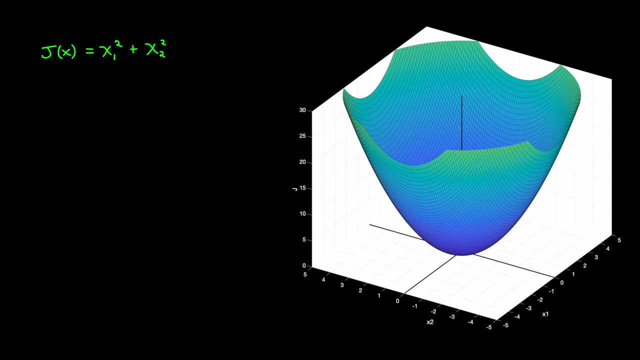 And the idea of looking at the slope can be expanded to higher order functions as well. For example, function j equals x1 squared plus x2 squared. We can look at this and once again pretty easily see that the minimum j occurs when x1 and x2 are both zero. Now to find this point, we once again look at: 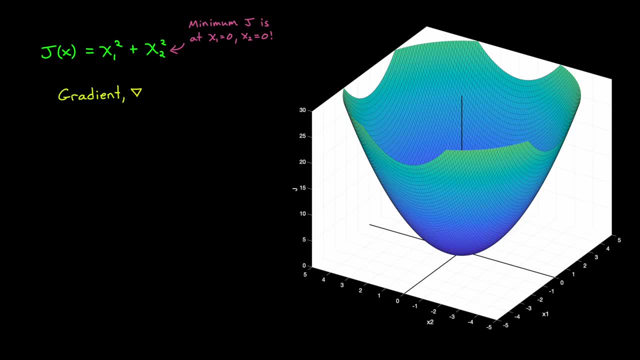 where the derivative is zero, or more precisely, where the gradient is zero. The gradient of j of x is the partial derivative of the function with respect to both x1 and x2.. And when we do this, we get the vector 2x1 and 2x2.. 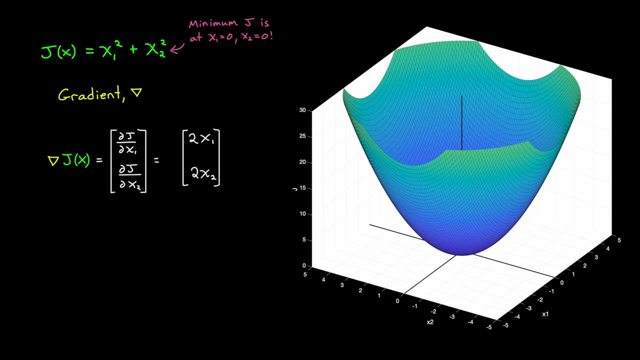 So really, the gradient returns a vector field that denotes the direction and the magnitude of the steepest slope for every possible x combination And for our bowl shape function the gradient looks like this: There is zero slope at the very bottom of the bowl, and then it gradually becomes. 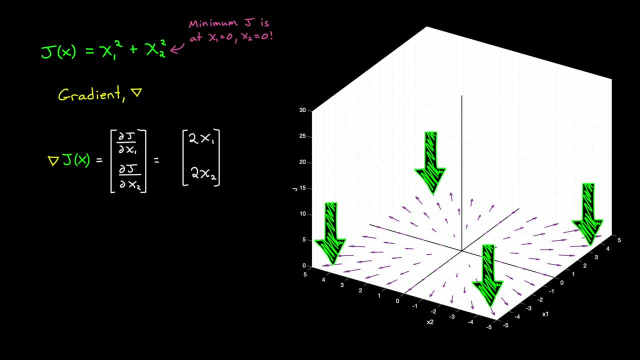 steeper as we move towards the edge in all directions, And this is the basis of all optimization problems. We set up an objective function and then solve for or in a lot of cases we search for locations of zero gradient. and i say search for because often objective functions aren't. 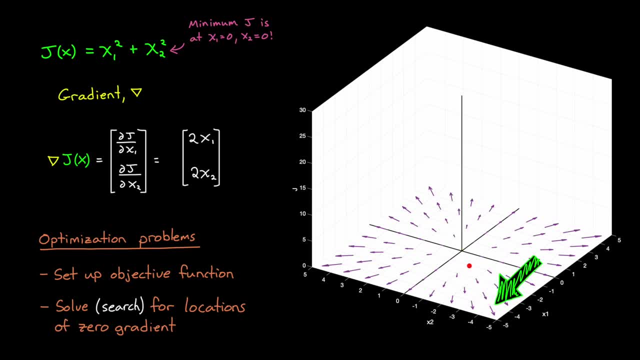 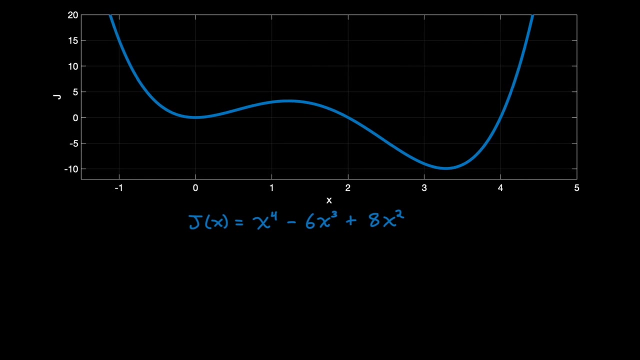 as straightforward as this, and we have to hunt for the optimal point with gradient descent type algorithms, and these are algorithms that find the optimal point numerically, with an iterative approach, by descending the gradient, that is, it's going in the opposite direction of the arrows until you reach a stationary point. all right, this is probably a good time to bring up the issue of 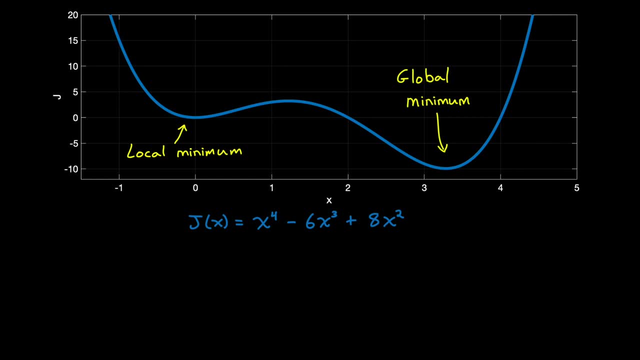 local and global minima. if we're looking for stationary points using gradient descent, then where that algorithm starts at search becomes really important. if there are multiple basins, then a gradient descent algorithm will get stuck in a local minimum if the starting state is within that basin of attraction. and there's different methods for addressing this, including just picking. 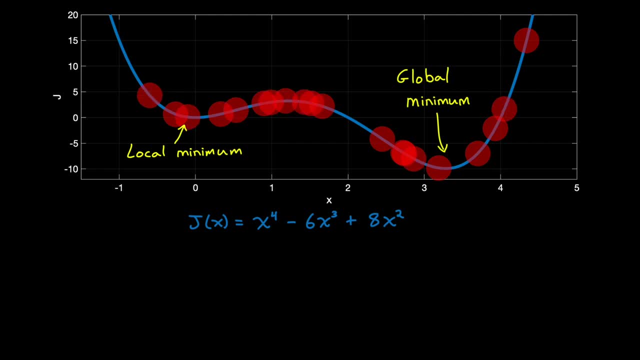 many different starting points and then using gradient descent to find the optimal point number points and then running gradient descent on each one and seeing where they all end up. but what's really nice about the analytical approach of taking the gradient of the function is that each of the stationary points can be identified mathematically. 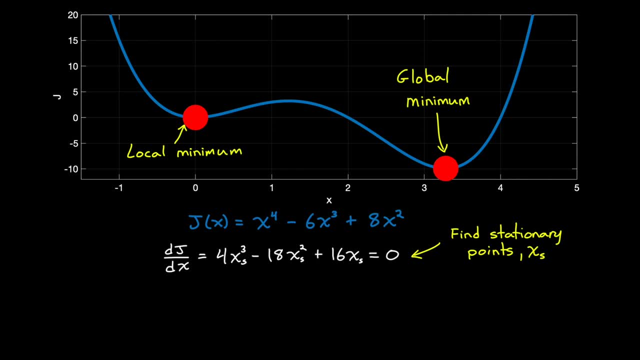 by setting the gradient to zero and solving for x. here we have three stationary points corresponding to the local minimum, the global minimum and the local maximum that occurs between them. so now we can just check the value of the objective function at each of these stationary points and then pick the lowest one to find that global minimum. 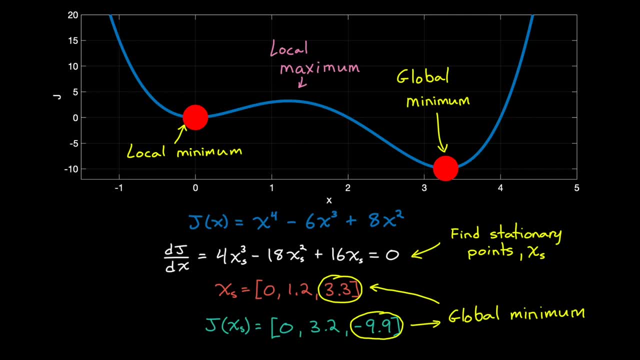 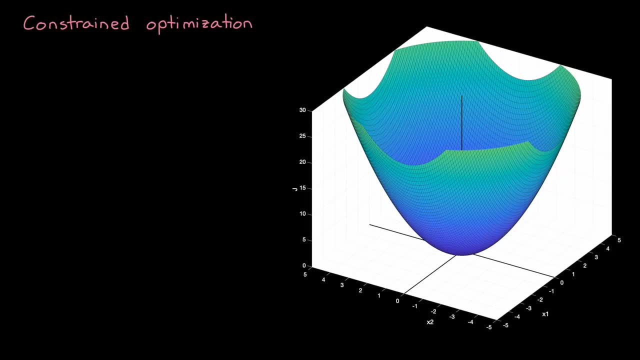 all right. so that's the unconstrained optimization. that's where we're free to choose any value that minimizes our function. but this video is on constrained optimization, and with constrained optimization, the objective function is subject to an additional constraint. in this case, let's say that the constraint is: x1 plus x2 plus 3 must equal zero, so that means that 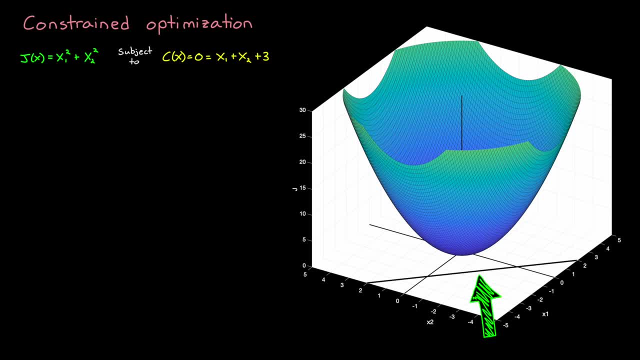 we can only choose the value of the objective function at each of the stationary points, choose combinations of x1 and x2 that lie along this line. And now, if I raise this line up, this means that we're really looking for the minimum value along this intersecting parabola. So now, how do we find this location? Well, let's. 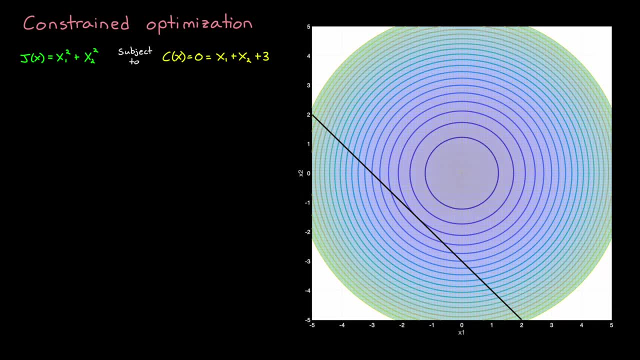 change the surface plot into a contour plot, And so now we can imagine that we're hiking along this black line on a surface that has this contour, And so at the beginning you're hiking down pretty steeply as you cross the contour lines quickly, and then it gradually gets less steep. And then right here, right when 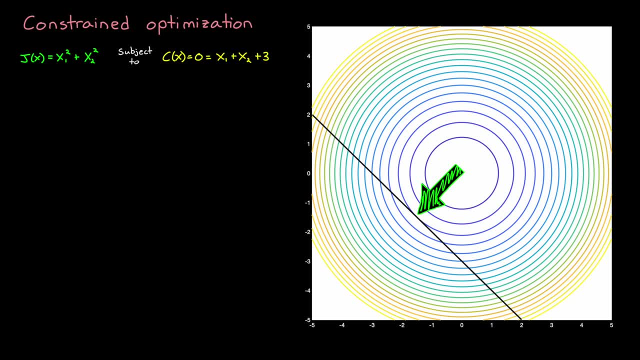 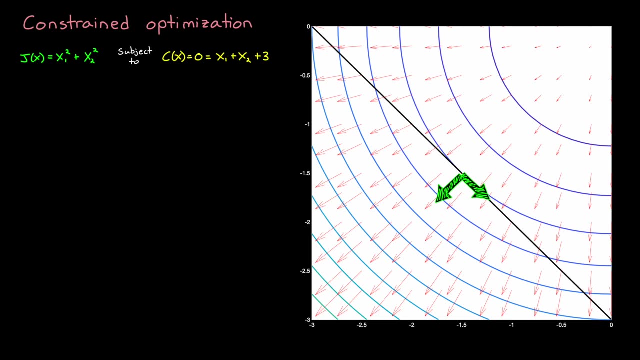 your path is exactly tangent to a contour line. you've reached the lowest point and then you know you start heading back up again. So the lowest point is where the path is parallel to the contour, Or another way of putting it, it's where the path is perpendicular to the gradient, And this makes sense, right? 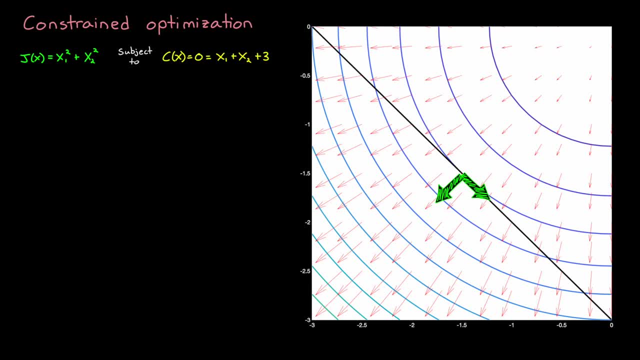 I mean, if the gradient is the direction of the steepest travel and you're walking perpendicularly to that, then you're not going up or down. So if you're walking perpendicular to that, then you're not going up or down. Right at that point your path is flat. Now to calculate this point, we can do. 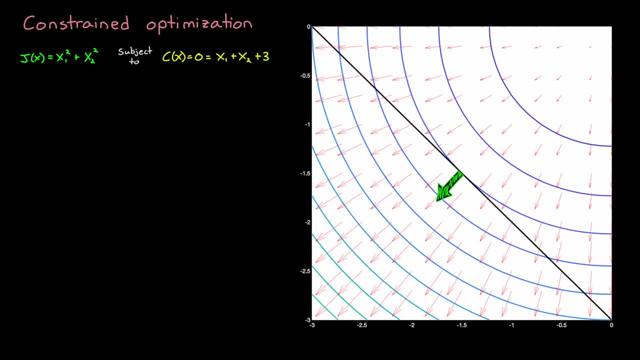 something clever, We can compare the gradient of the objective function with the gradient of the constraint, And if the gradients or the directions of the steepest slope for the two functions are parallel, then this is a stationary point And therefore it's either a maximum, a minimum or some kind of a saddle point. 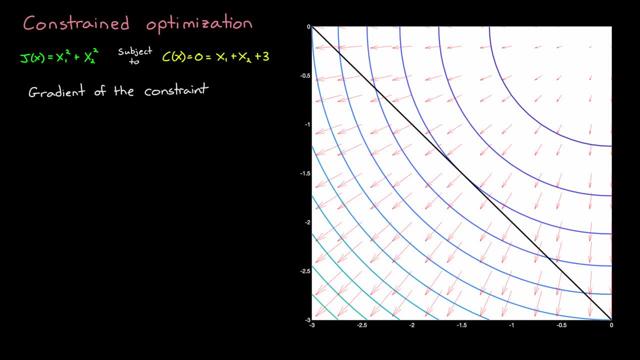 like we had with x cubed. So the gradient of the constraint is the partial derivative with respect to both x1 and x2, which it turns out is just one for both directions. And if I plot that vector field on our graph, we get these arrows that are all perpendicular to the black line, And notice that at the 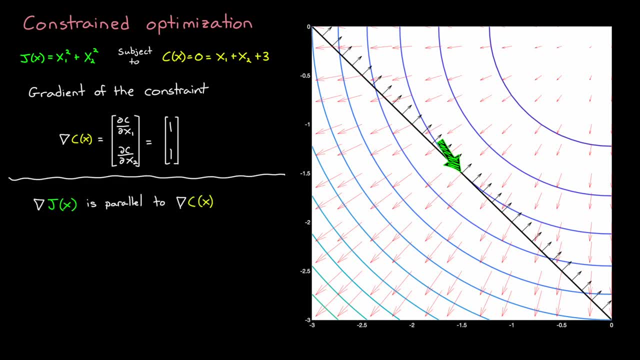 minimum point, the gradient of J is parallel to the gradient of C. Now they are pointing in different directions, but they are parallel. So to make them equivalent we can simply multiply the constraint by a constant lambda, And choosing different lambdas is essentially scaling the gradient. you know, either positively or negatively. 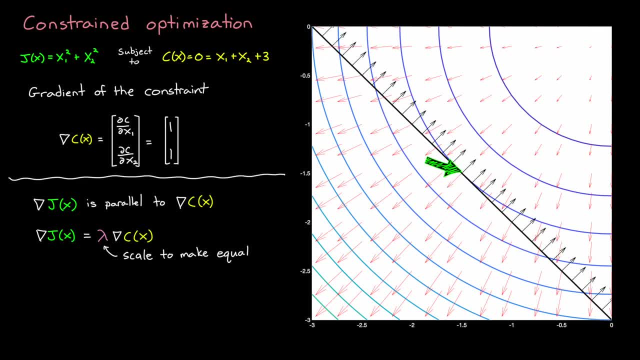 like I'm showing here, And the idea is that we want to find the Lagrange multiplier that makes the two gradients equal right at this point where they are parallel. Okay, so now let me rearrange this equation, and what we're left with is the equation that we started with. Now you're gonna notice that if you do this. 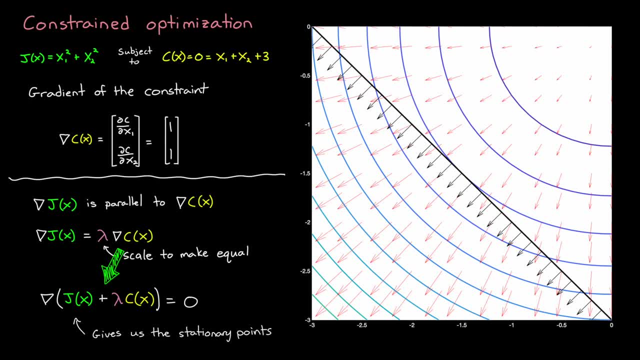 rearranging yourself a minus lambda c. but to make the equation look better, we just roll that negative into the constant lambda, which can be positive or negative. All right, so the solution to the problem exists where the gradient of the Lagrangian equals zero, And again, this doesn't tell us if we're at a. 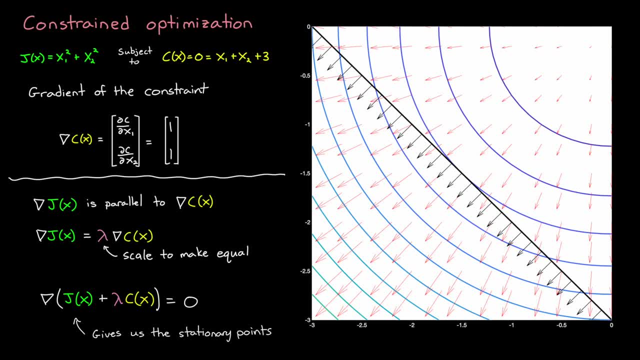 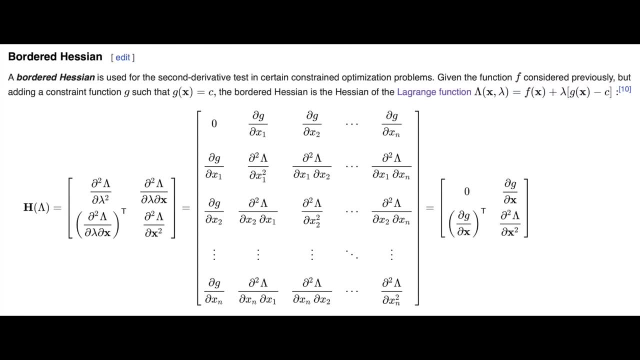 maximum, a minimum or a saddle point. We know that we need some form of a second derivative to determine that And, generally speaking, that second derivative comes in the form of a bordered Hessian matrix, And I'm not going to cover this here, since I just wanted to talk about the. 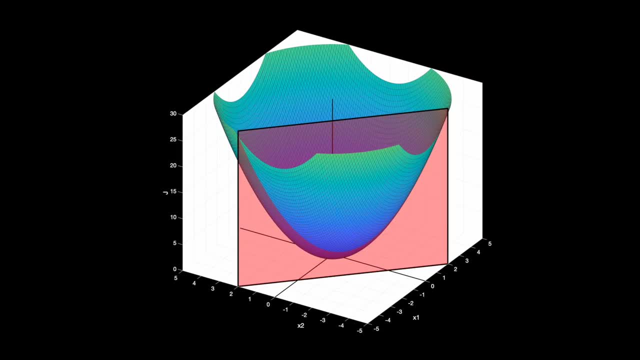 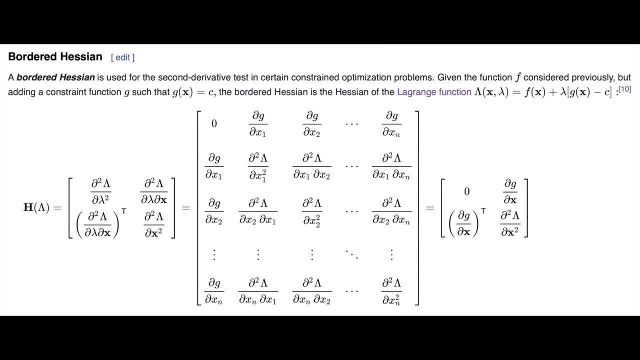 Lagrangian itself And also in our problem. we know that the point is a minimum due to our understanding of the functions, But I did leave some good references for it down below All right, so now that we understand why the Lagrangian is important, let's use it to solve the constrained. 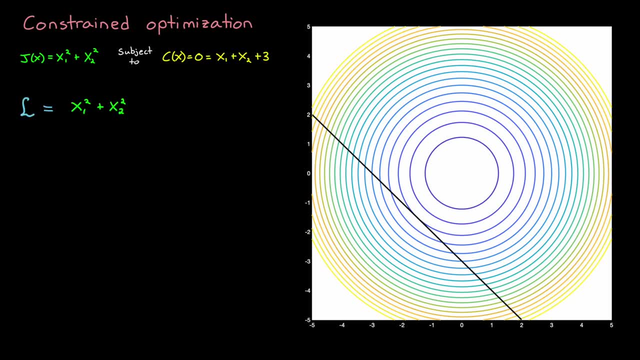 optimization problem. Our Lagrangian is x1 squared plus x2 squared plus lambda times x1 plus x2 plus 3.. And the gradient gives us these three equations which we can use to solve for the three unknowns by just setting each of the. 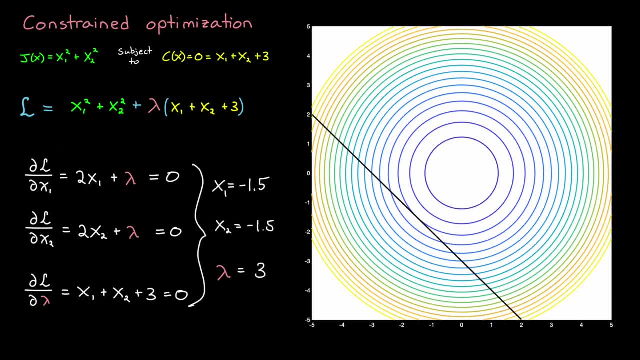 equations to zero And we find that the optimal point is at minus 1.5 and minus 1.5. And the Lagrange multiplier has a value of 3.. And how cool is that? I mean, it's just such a simple idea that. 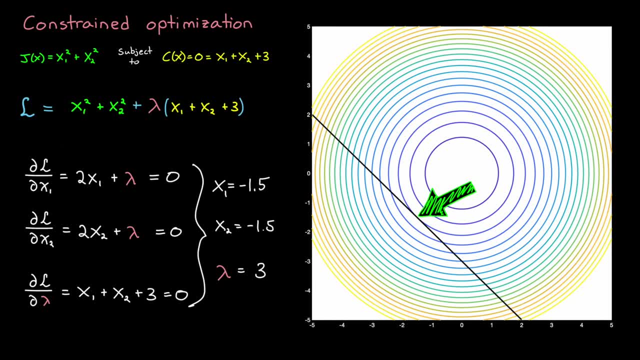 we can find minima and maxima. We can find maxima of constrained optimization problems just by looking at where the gradients of the two functions are parallel. All right, so now, before I wrap up this video, I want to show you how we can actually solve this example in MATLAB, since, more often than not, you're not going to be. 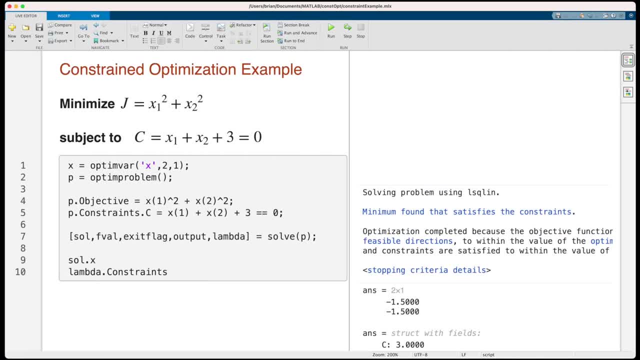 solving it by hand. I have this live script that uses the well-named function optimProblem to solve our optimization problem, And here I've defined the objective function: x1 squared plus x2 squared, and then the constraint: x1 plus x2 plus 3 equals 0. The function solve solves the problem and it 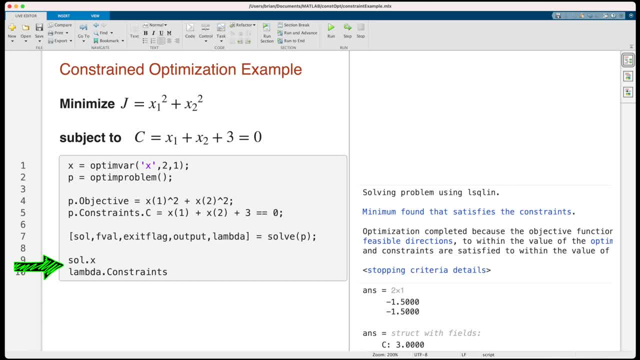 returns several different outputs And when it runs, I'm displaying the optimal point, x, and the Lagrange multiplier, lambda, And over here we see that x is minus 1.5 and minus 1.5, and lambda is 3, just as we calculated. All right, so that's where I'm going to leave this video, Hopefully. 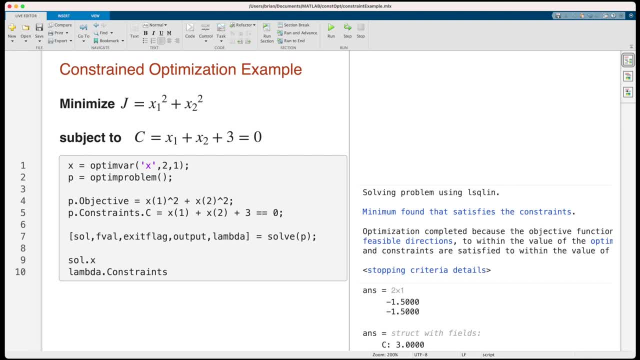 you have a better understanding of how the lagrange multiplier works. And if you have any questions, please feel free to leave a comment below. I'm going to be happy to answer any questions you may have And I'll be happy to answer any questions you may have. And I'll be happy to answer any questions you may have.